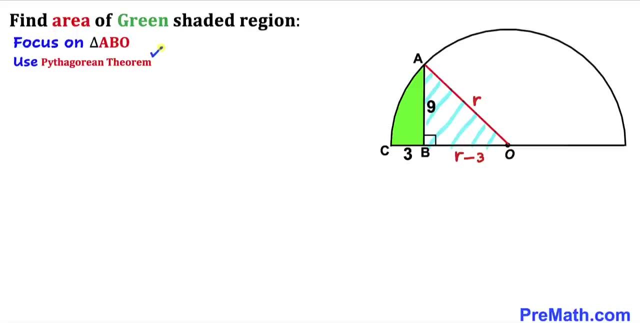 are going to use the Pythagorean theorem to solve for radius r. And here's our Pythagorean theorem: a square plus b square equal to c square. Let me call this longest leg as our side. See, I'm going to call this side lowercase a and this lowercase b, So let's go ahead and fill in the. 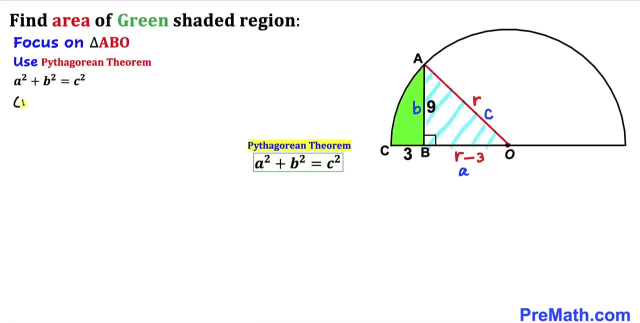 blanks in this Pythagorean formula. A, in our case, is r minus three. So this is going to become r minus three. whole square plus b is nine square equal to r square. And now let's recall this famous identity: a minus b whole square could be written as a square minus two ab. 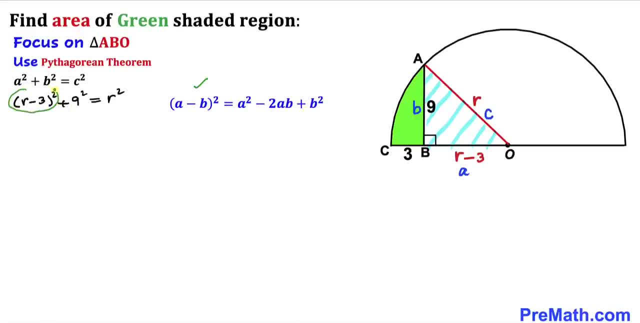 b square. We are going to apply it on this binomial on the left hand side. So therefore this is going to become r square minus six, r plus nine And nine square is going to give us 81 equal to r square. And here we can see: this r square cancels out with this r square on the right hand side And as a. 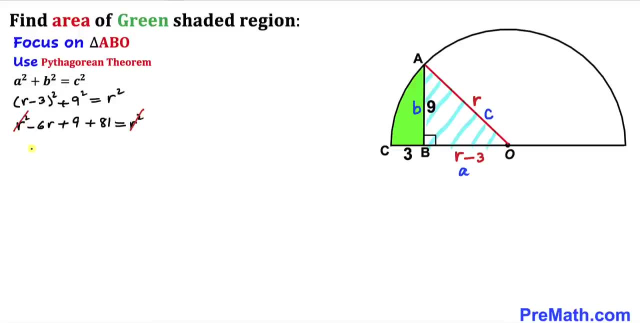 result: if we combine the like terms on the left hand side, We're going to get negative six r plus 90 is going to be equal to zero. Let's move this 90 on the other side. So therefore we are going to have negative six r equals to negative 90.. Let's 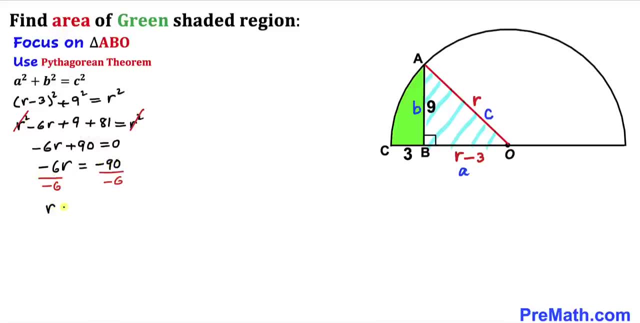 divide both sides by negative six. So therefore, our radius r turns out to be 15 units. So, therefore, this radius r turns out to be 15 units And, moreover, this side length of this triangle ob is going to be 15 minus three is going to give us 12 units. And now let's make an observation. we can see that 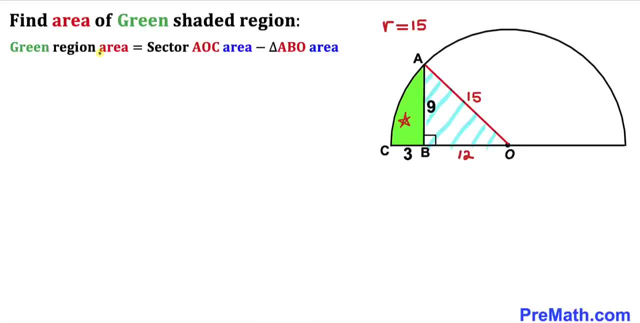 the area of this green shaded region is going to be equal to the sector aoc area, This whole sector aoc minus the area of this right triangle abo. So therefore, our task is to calculate the area of this sector aoc And also calculate the area of this right triangle abo. And here's: 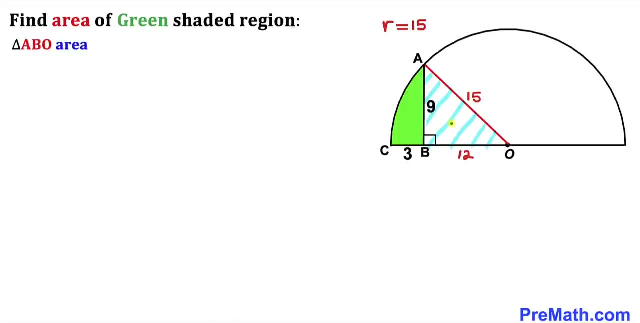 our next step. Let's go ahead and calculate the area of this right triangle abo. And now let's recall the area of a triangle formula: area equals three. And now let's go ahead and calculate the area of a triangle formula: area equals three. And now let's go ahead and calculate the area of Military. 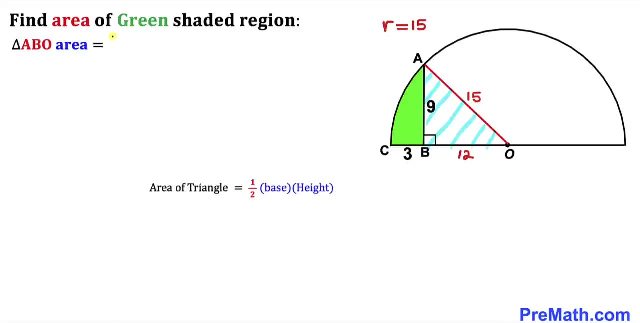 피 Hepatosコンム iiones at spot dot 0. Then is equal to the area of this right triangle abo. So here I also want to calculate the area of this right triangle abo, And if the area of this right triangle abo is critical, the area of this right triangle is egal, so it will also be her. 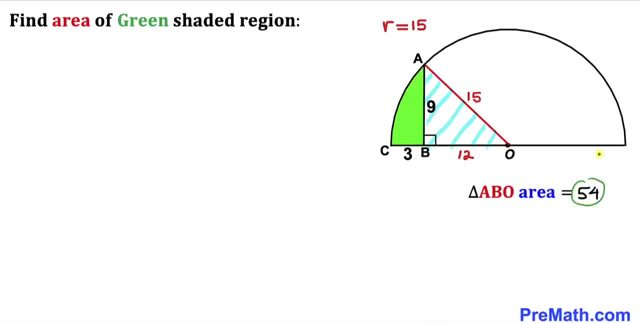 ABO turns out to be 54 square units. and now let's focus once again on this triangle ABO. and now let's recall the Pythagorean triplets 3, 4, 5. and if we multiply all these numbers by 3, then our new Pythagorean triplets is going to become 9, 12 and 15, and that's what we got. 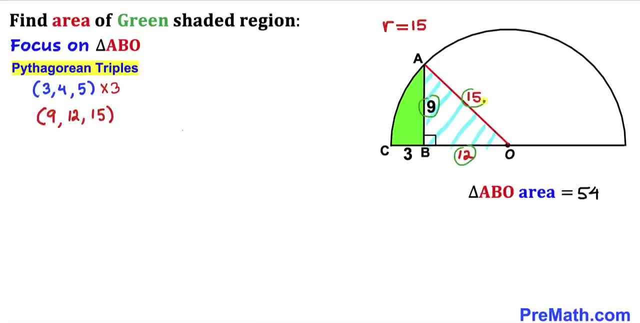 as our side lengths of this right triangle. and here I have copied down this right triangle, ABO, whose side lengths are 9, 12 and 15. and in such kind of right triangle this is our smallest angle, since this is opposite to this smallest side length. and in this triangle this angle has got. 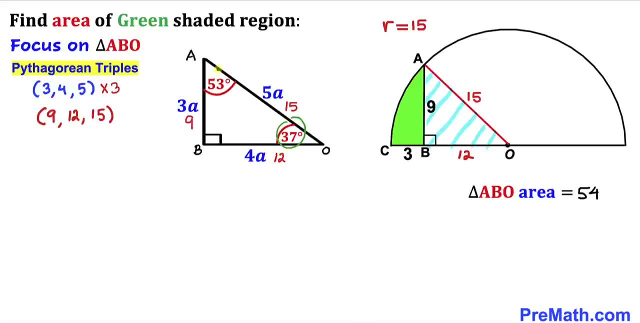 to be 37 degrees And this angle has got to be 53 degrees, and this is going to be our 90 degree angle. So therefore, we conclude that this angle is going to be 37 degrees, and let me show you the alternative approach to calculate this angle: BOA. and now let's recall SOH CAH TOA. 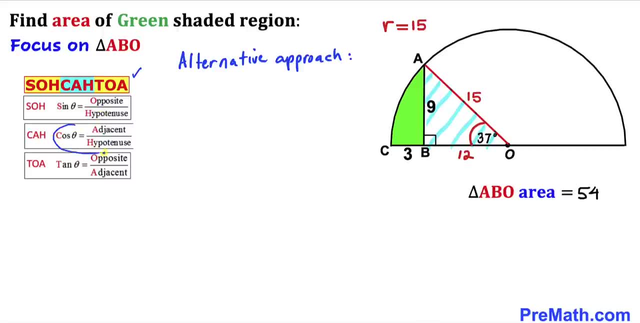 and we are interested in cosine of theta equal to adjacent divided by hypotenuse. If I call this angle as theta and this is our adjacent side and this is our hypotenuse, then our cosine of theta is going to be equal to 12 divided by 15 and the right hand side. 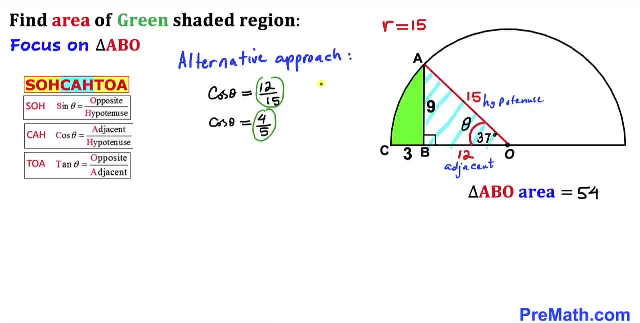 12 divided by 15 could be reduced to 4 fifth. so therefore, angle theta is going to be equal to cosine inverse of theta. So this is our hypotenuse angle. So if I call this angle as theta, and this is our adjacent side and this is our hypotenuse. 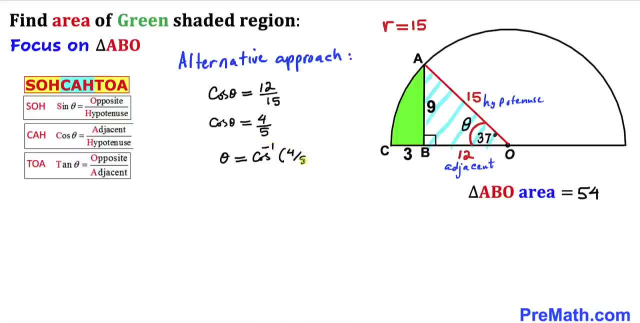 So this angle of theta higher than equal to is equal to 30 degrees to the cube. and now let's recall over here the bus angle, mountain angle of theta greater than 0. So this is the angle theta higher than 1.. So this angle theta is equal to assets of that factor. 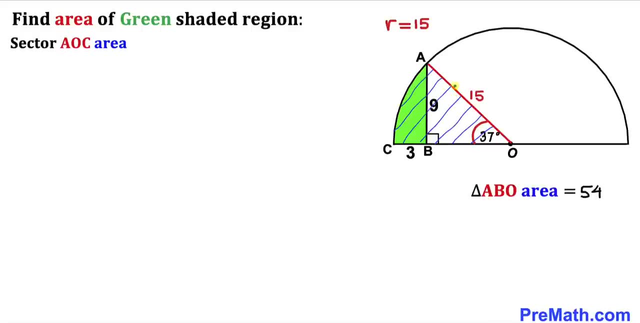 So let me give a quiz again. let's calculate the area of the sector AOC. So in our denominator of this personal data we can write: we have that A through sigma, plus B plus A over here. Okay, angle theta divided by 360 degrees times pi r squared, and in our case our angle theta is: 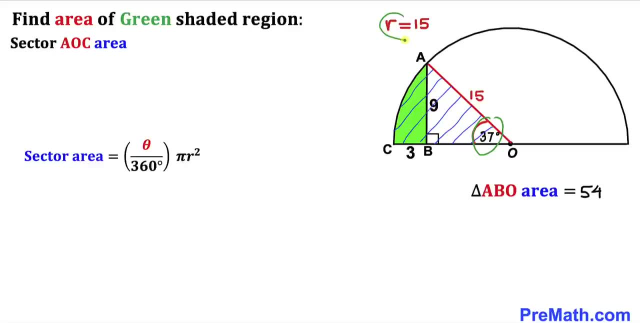 37 degrees and our radius is 15.. So therefore, the sector area is going to become 37 degrees, divided by 360 degrees times pi and r, in our case, is 15 whole square. And here in the next step, 15 square gives us 225, and if we simplify everything on the right hand side, that has 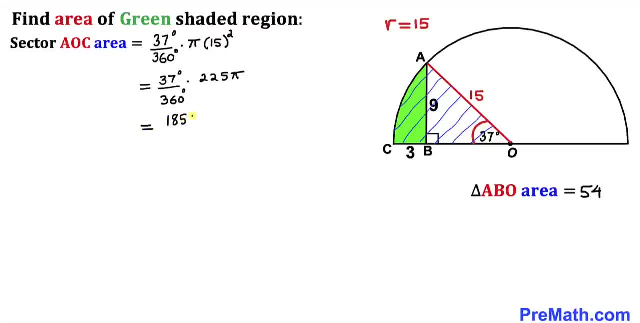 got to give us 185 pi divided by 8.. and here's our final step. let's go ahead and calculate the area of this green shaded region. we already figured out this sector AOC area, which is 185 pi divided by 8, and the area of this. 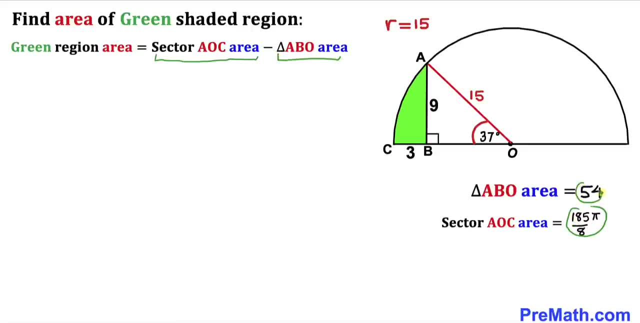 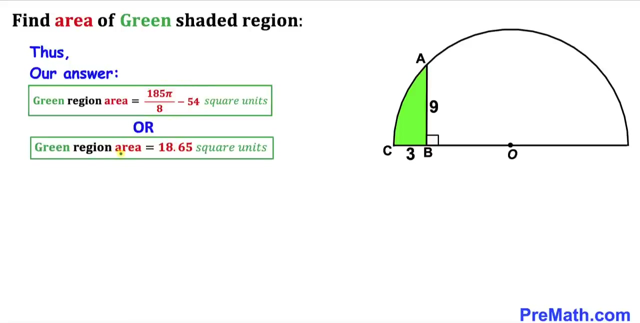 triangle ABO is 54, so therefore the green shaded region area is going to become 185 pi divided by 8 minus 54, and here's our final answer, as you can see over here. and this green shaded region area could also be written as equal to 18.65 square units. 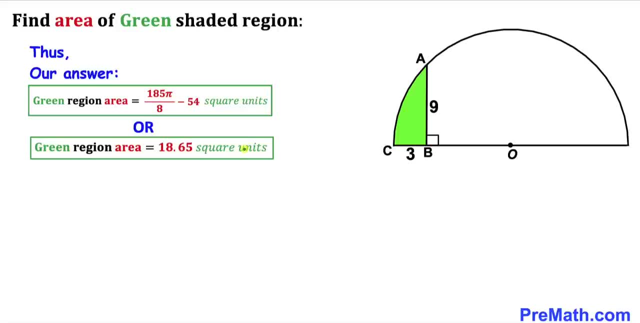 thanks for watching and please don't forget to subscribe to my channel for more exciting videos. bye you.